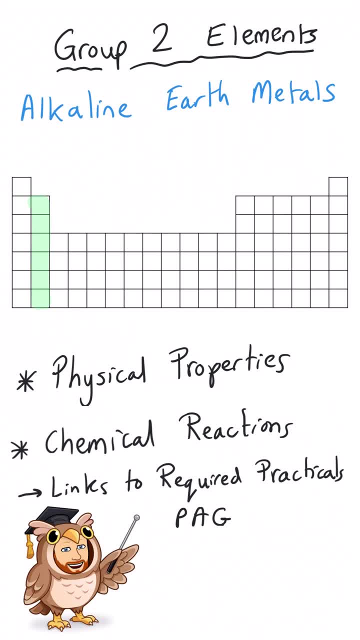 Hello everybody and welcome back to the channel. I'm here with a video about the A-level chemistry topic, group 2 elements. So this is the alkaline earth metals which is the green column of the periodic table. I've shown here, Typically topics like you to look at the elements from magnesium. 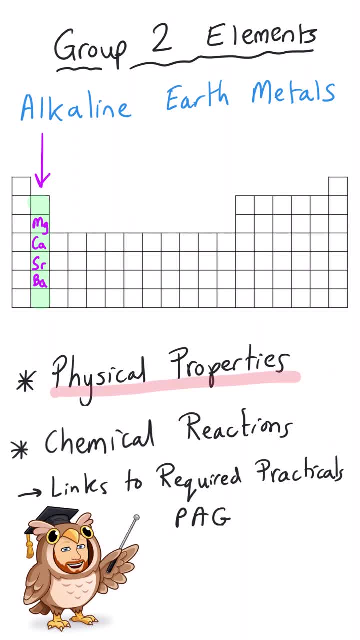 to barium, but we're going to talk about the physical properties generally and the chemical reactions that these elements undergo. This has strong links to the required practical number 4 if you take AQA A-level and the PAGs for OCR and for practical assessments generally. 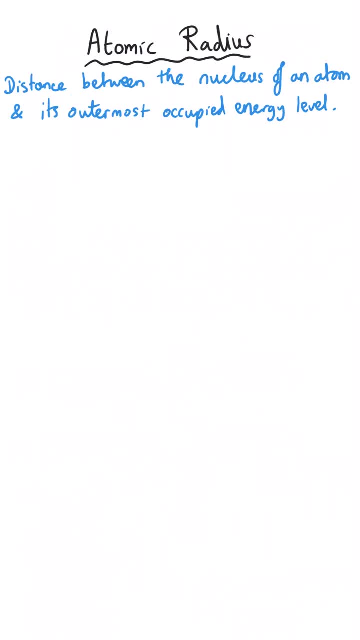 The atomic radius of an atom is a measure of the amount of space that that atom occupies, and so a larger atom will have a larger radius. The size of the atom, then, is determined by the number of occupied electron shells, or energy levels, that that atom has got, and so 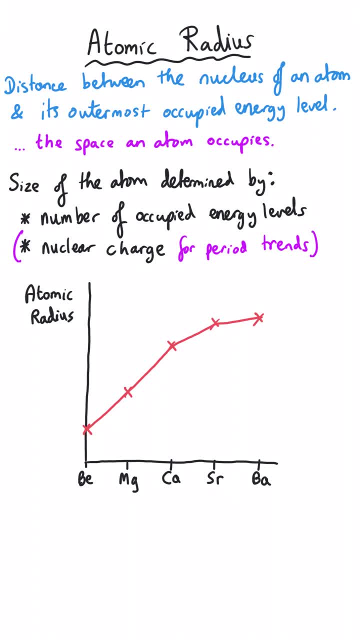 as you go down group two in the periodic table, the number of occupied energy levels increases by one each time, And so, as a result, the atomic radius goes up. It's not a perfectly linear pattern, and you don't need to worry about all the particular nuance. You just 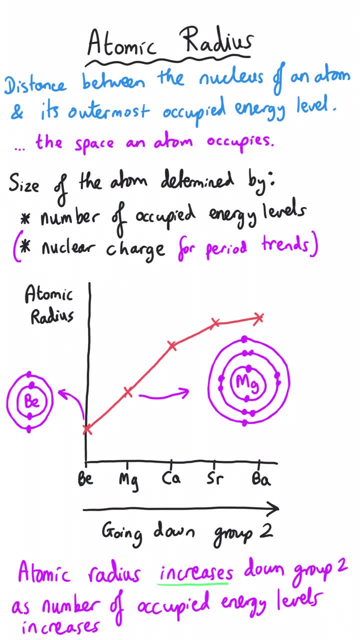 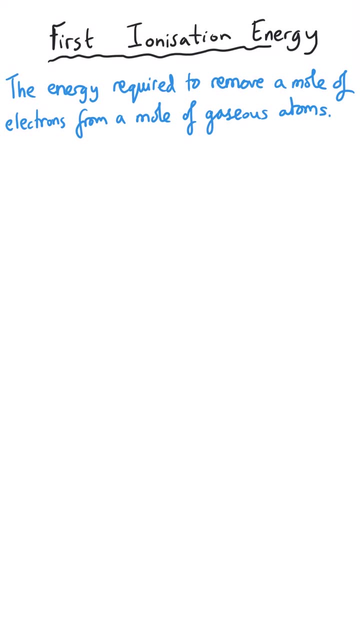 need to know that that atomic radius increases as we work our way down the group, from magnesium to barium, And that pattern would continue outside that range as well. The first ionisation energy for an atom is a measure of the amount of energy that's. 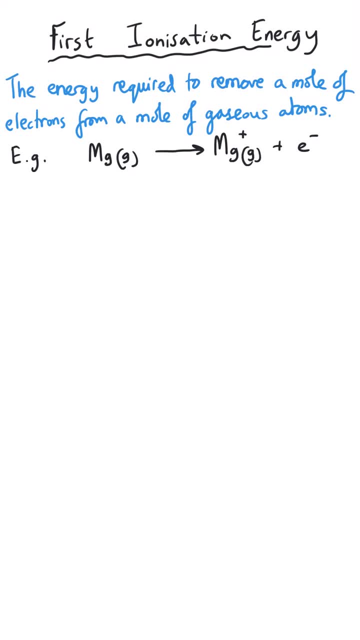 required to remove a mole of electrons from a mole of gaseous atoms And how much energy is required to do this depends on the strength of attraction that that electron is experiencing from the nucleus. The larger the nuclear charge, the stronger the attraction between the nucleus. 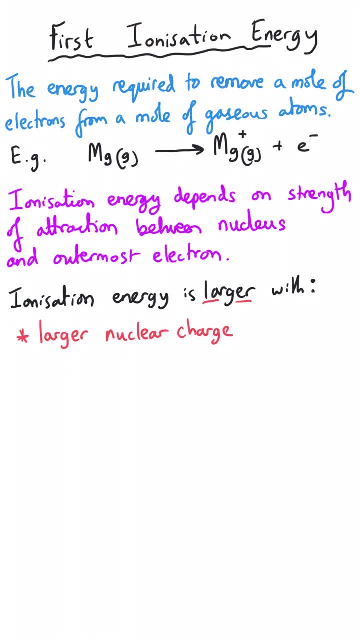 and the outermost electron, the more energy will be required to remove that electron. Additionally, the greater the distance between the nucleus and the outermost electron, the smaller the ionisation energy will be, because that electron is experiencing a weaker pull. As a result of this, it is easier to remove an electron from a larger atom in group two. 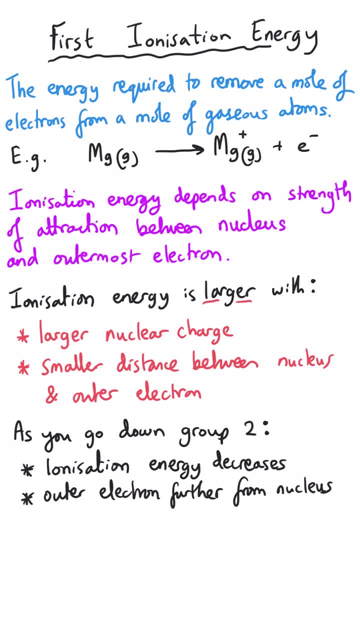 And so, as we work our way down group two in the periodic table, the barium atom, for instance, which is the furthest one down that we go to in this pattern, is much smaller than the strontium and calcium and magnesium, for instance, and therefore it is much easier. 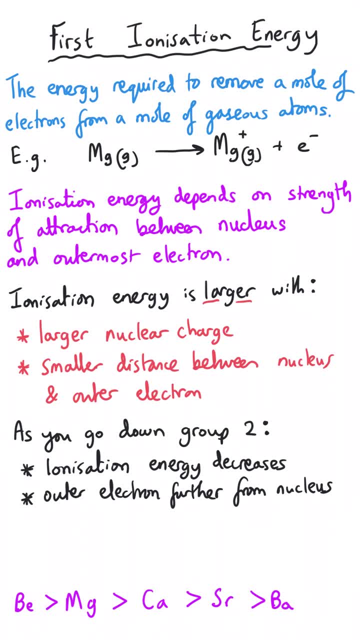 to remove the electron from the atom because the nucleus' pull is being shielded by all these additional energy levels between the nucleus and the outermost electron. So it is much easier to ionise the atom as you work your way down the group. 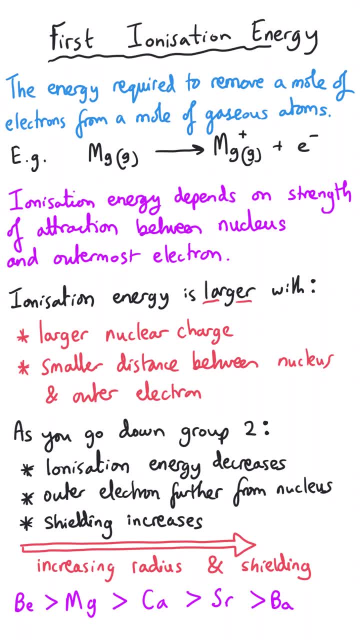 This pattern shows that it is the shielding and the number of occupied energy levels that are required to remove the electron from the atom. This pattern shows that it is the shielding and the number of occupied energy levels that are required to remove the electron from the atom and the atomic radius that are more significant. 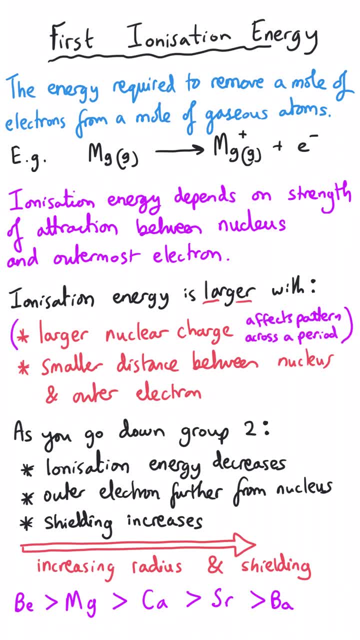 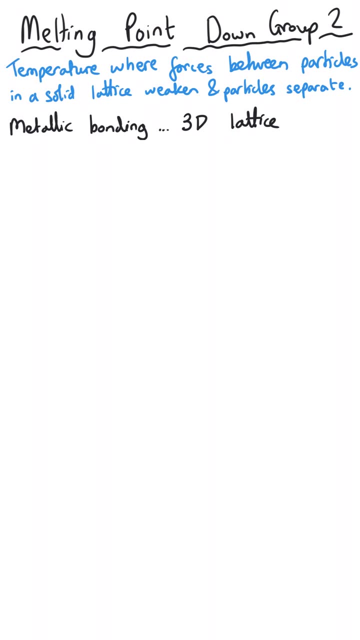 than the nuclear charge, because this decrease in ionisation energy happens in spite of the increased nuclear charge in the nucleus. The group two elements are metals. they are the alkaline earth metals and what that means is that their structure is a crystal structure of a three-dimensional lattice of 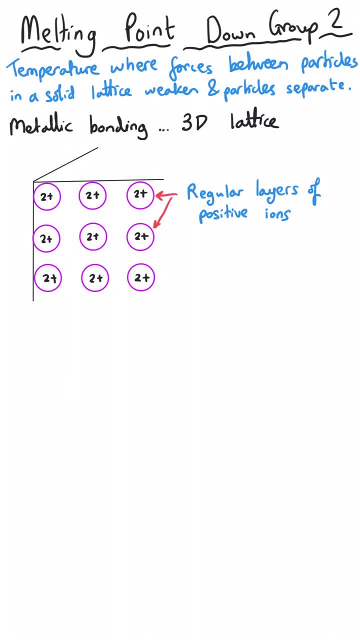 metal ions, in red and in blue, in regular layers with delocalised electrons moving between them, And this is what gives them their properties of high melting point, malleability etc. Because they're all in group two. there are two delocalised electrons per atom or per ion as it becomes, And they all become. 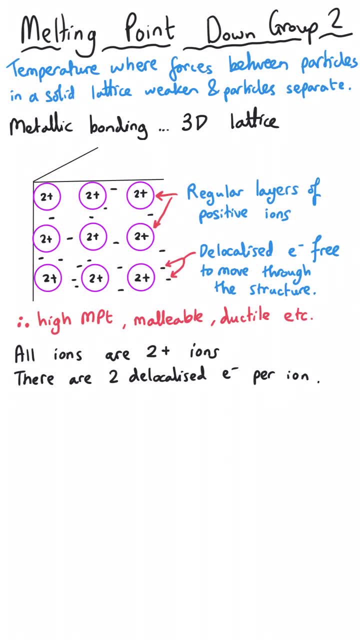 2 plus ions, And so they all have a 2 plus charge. However, as we know, the radius gets larger as we go down the group, And so that means that that charge is spread over a bigger area or a bigger volume really, And so that means the charge density is going to decrease as we go down the 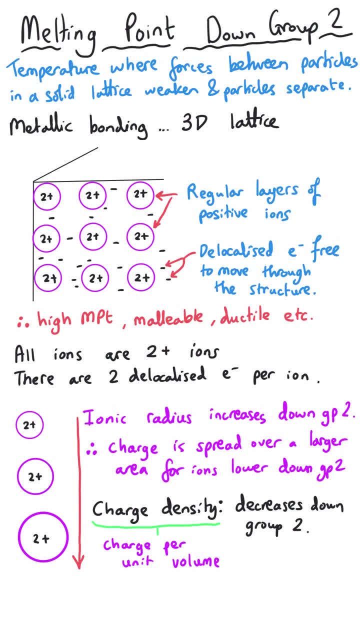 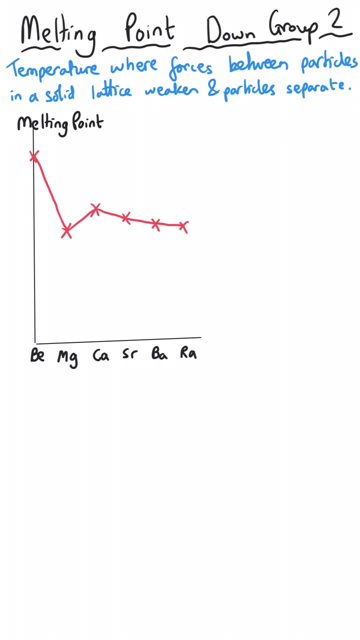 group because the charge is spread over a bigger area. As a result of that, the charge density will decrease and the delocalised electrons that are within the lattice will experience a weaker attraction for the ion itself. So if we were to compare something like calcium, calcium's melting. 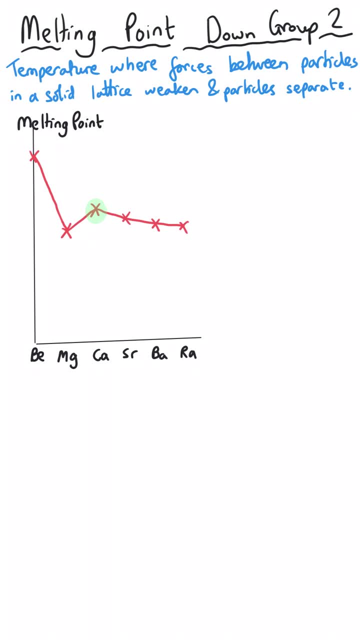 point will be higher than the melting point of barium, because there is a larger charge density for calcium, And so there is a greater attraction for the delocalised electrons to the calcium ions, And so more energy is going to be required to break this. 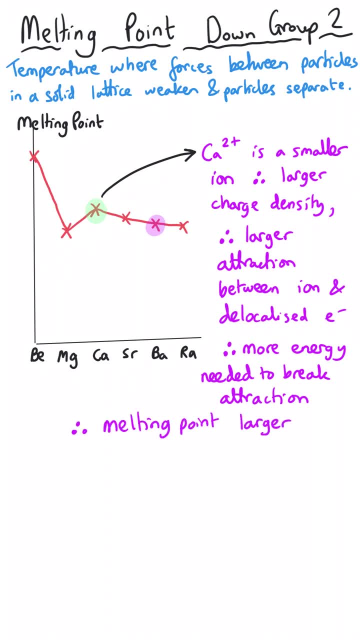 attraction, and so there is a greater attraction for the delocalised electrons to the calcium ions, And so more energy is going to be required to break this attraction, and therefore the melting point of calcium will be greater than the melting point of barium. 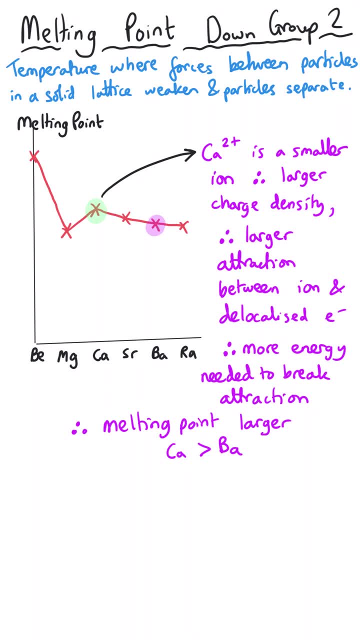 And so that is a general decreasing pattern as we work our way down group 2.. It's not always a decrease by the same amount. The actual crystal structure is slightly different from one metal to another, but that general pattern is something that you need to know. 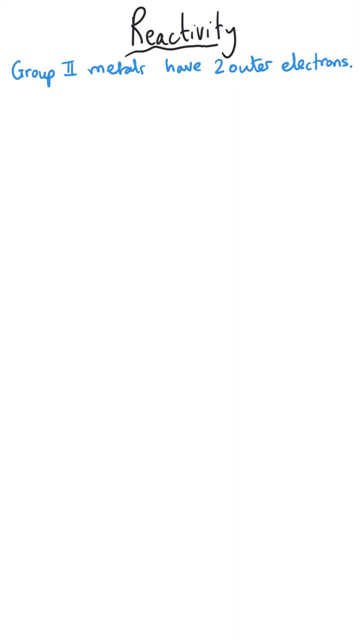 If we take a look at some of the reactions of the group 2 elements, we first need to consider the reactivity. When the group two elements react, they always react in a predictable way and that's because their goal through reacting is to become more stable, and the way that elements 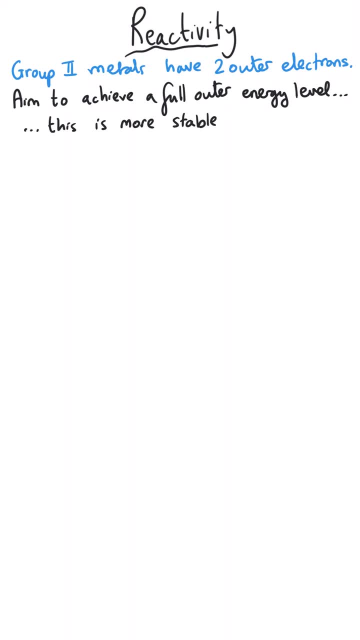 become more stable is they achieve a full outer occupied energy level of electrons. and since the group two elements have two electrons in their outer energy level, they need to lose those two electrons in order to become stable and have a complete inner energy level. So the reactivity of 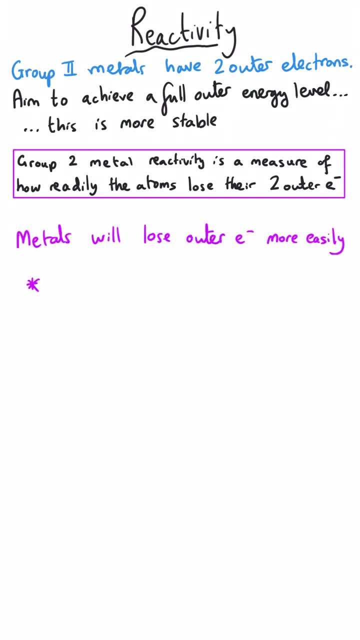 the group two elements is influenced by how readily they will lose those two outer electrons and then in a similar way to ionization energy. that means that the larger the element is, the weaker the attraction will be from the nucleus to the outer electrons that are being lost and that 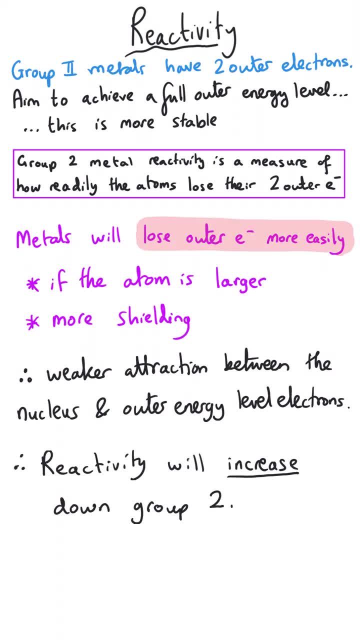 means that they will be lost more easily And so they will be more reactive. and so you find that the reactivity will increase as we go down the group because of the increased atomic radius, the increased shielding and therefore the weaker force of electrostatic attraction that the outer electrons experience from the nucleus, and so less energy is needed to remove those electrons, and so they 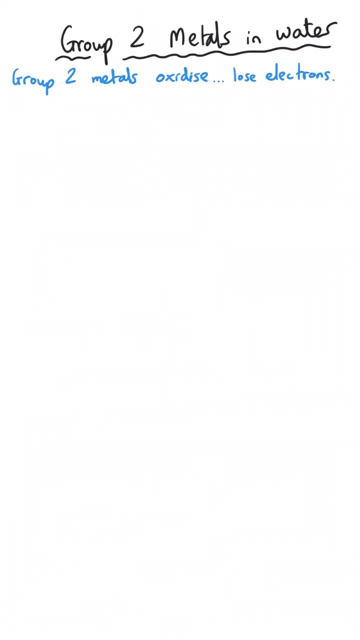 become more reactive. You can prove the pattern in reactivity of the group two elements by looking at how they react with water. As we know, the group two elements react by giving away their two outermost electrons in their outermost occupied energy level. This is an oxidation reaction, because the elements have lost electrons and so, in general, the element itself starts with an oxidation state of zero and it gives away two electrons, which leaves the metal with an oxidation state of plus two. 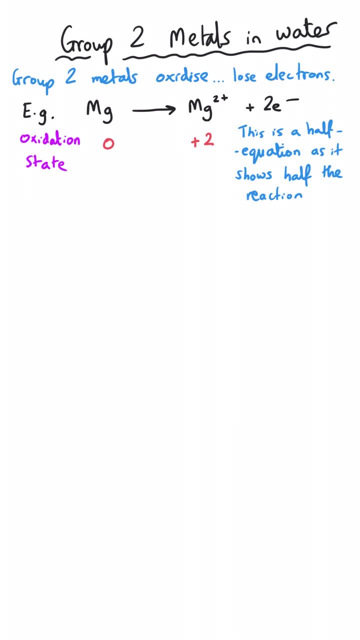 For instance, magnesium turning into magnesium two plus, that means it must have lost two electrons, and so we put those two electrons on the right hand side with the rest of the products. So when the group two metal reacts with water, the metal gives away two of its electrons to the water. that is reacting specifically to the hydrogen atoms in the water, because the hydrogen atoms in water begin with an oxidation state of plus one and they finish with an oxidation state of minus one. 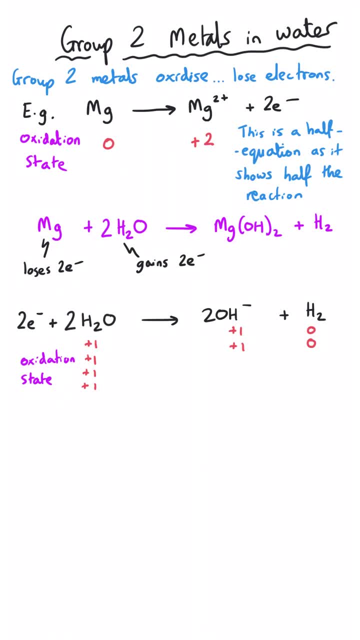 with an oxidation state of zero, or at least the two that go on to become hydrogen gas do, And so that means that this is a redox reaction, where the fizzing is produced by the hydrogen gas, and this hydrogen gas has been reduced. it has gained electrons from the magnesium. 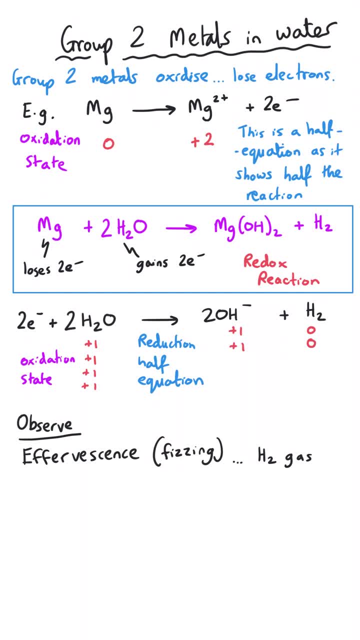 And so, in general, whenever a group two metal reacts with water, we will see fizzing from the hydrogen gas that is being produced, and we will note that the solid is disappearing as it reacts, and so that piece of magnesium, for instance, will get smaller, And so this is the overall equation. 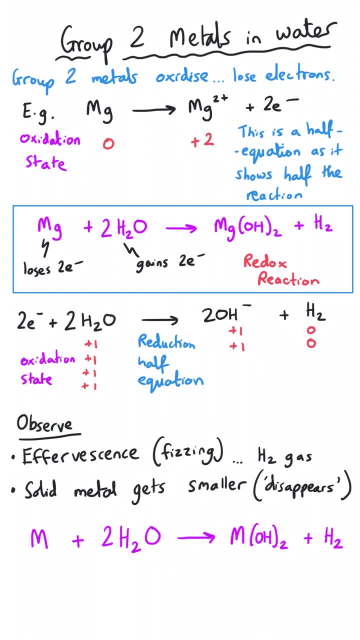 Metal plus two water turns into metal hydroxide and hydrogen gas. In the case of calcium, for instance, it's calcium solid water is a liquid, calcium hydroxide is aqueous and hydrogen is a gas, But as we will explore later, 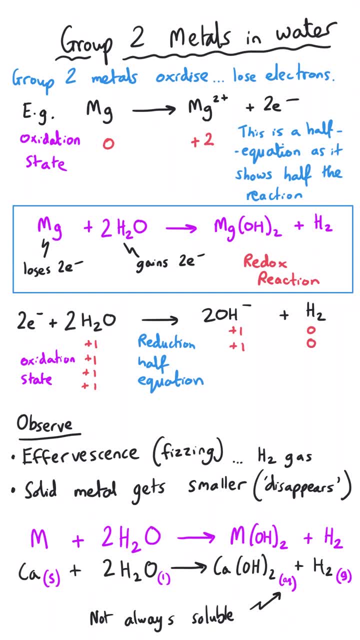 the hydroxide is not always aqueous, Sometimes it is solid. The group two metals become more reactive as you work your way down the group. So, for instance, beryllium does not react with water, Magnesium is very, very slowly with cold. 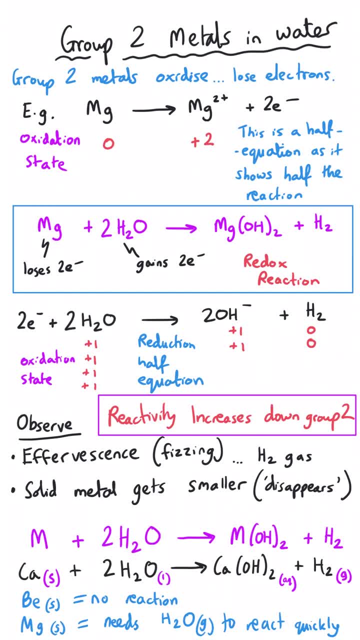 water. It needs really to be steamed to make it react impressively. Calcium is faster, then strontium and then barium is a very rapid reaction indeed to produce barium hydroxide and hydrogen When you form metal hydroxide. 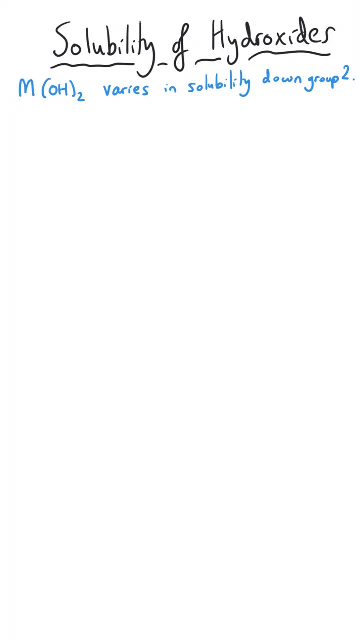 for instance, after a group two metal has reacted with water, the hydroxides themselves will have a different solubility depending on what the group two metal was. There is a pattern as we work our way down the group that hydroxides get more soluble the larger the group two element is. 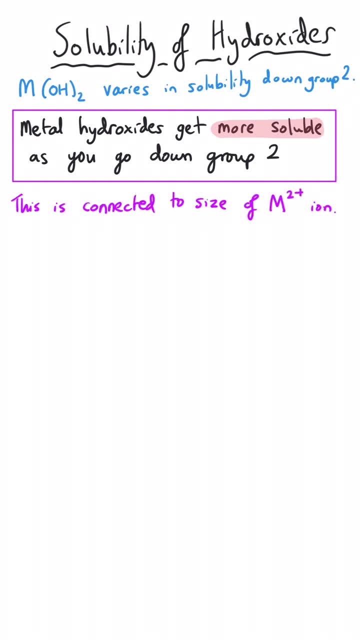 more specifically, the larger the group two ion is: Magnesium hydroxide is actually the least soluble hydroxide in the group And if you carry out a chemical reaction where you produce magnesium hydroxide, you will know this because you've made a white precipitate. So, for instance, 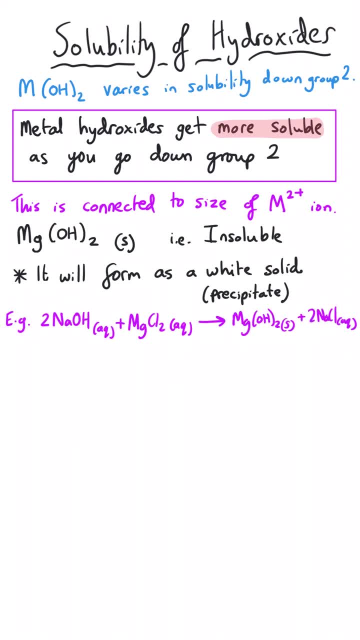 if you add sodium hydroxide to a substance that you think contains magnesium ions, the formation of a white precipitate is supporting evidence that that indeed was present. The ionic equation for this is magnesium ions, aqueous two plus react with two. 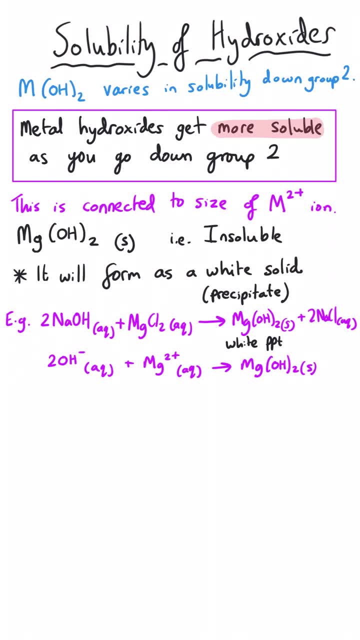 hydroxide ions also aqueous and they produce the magnesium hydroxide solid, which is the white precipitate that we observe And that is utilised in antacid remedies, indigestion remedies, where you might take some magnesium hydroxide and that would neutralise the acid in the stomach. Calcium: 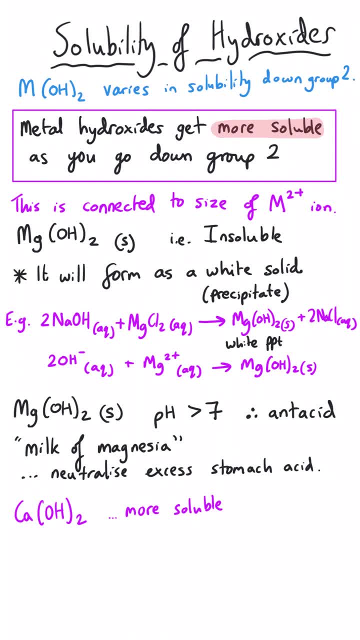 hydroxide is much more soluble than magnesium and it is used in agriculture as something called slaked lime, where its alkaline properties are utilised to neutralise acidic soil to raise the pH for growing a particular crop. Once we get to strontium and barium, these hydroxides are fully 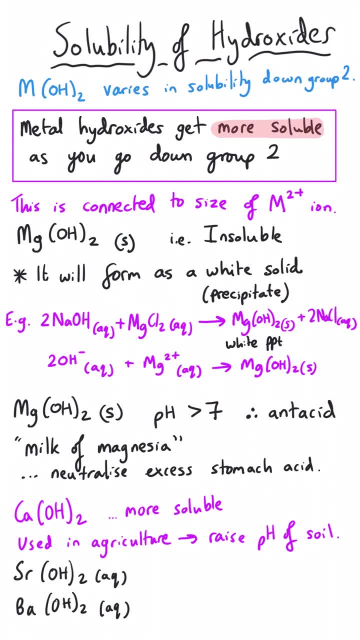 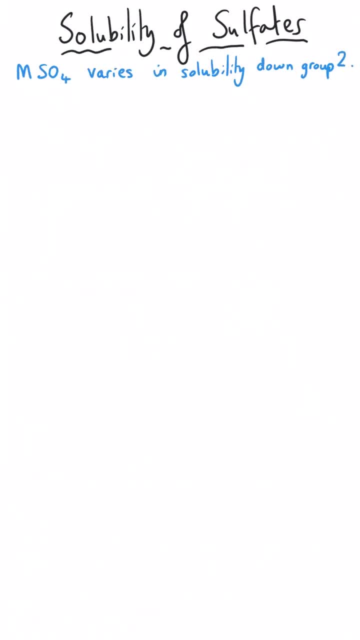 soluble and you will never get a precipitate during the formation of a barium hydroxide compound, for instance. Group 2 metals react with compounds containing sulphate to make metal sulphates. You need to know that the sulphate is a solubility of these sulphates changes as you work your way down. Group 2, with magnesium sulphate. 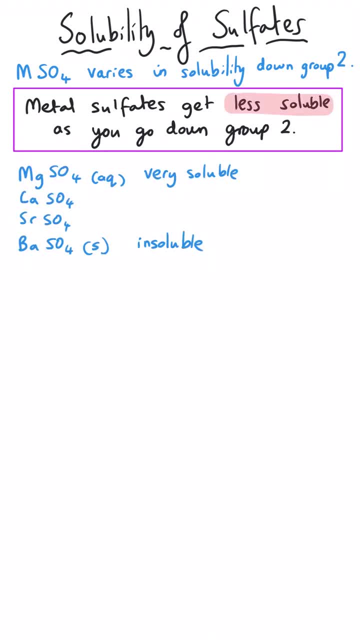 being very soluble and then barium sulphate being the least soluble, And it's a pattern of solubility increase as we go up the group. This can be utilised when we're trying to test for the presence of either sulphate ions or barium ions in a solution. So if we've got a solution, 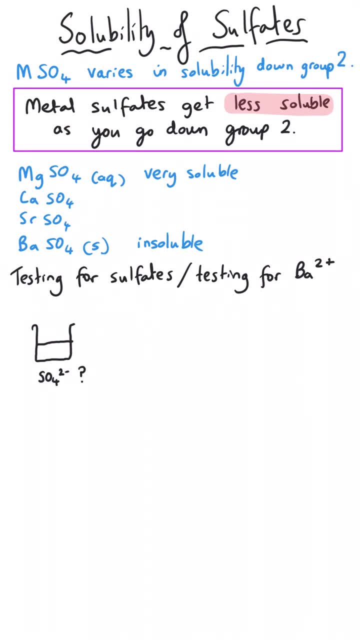 that we think might contain sulphate ions, we're going to need to test for the presence of either sulphate ions or barium ions in a solution. So if we've got a solution that we think might contain sulphate ions or barium ions in a solution, we can add something to it, such as barium chloride. 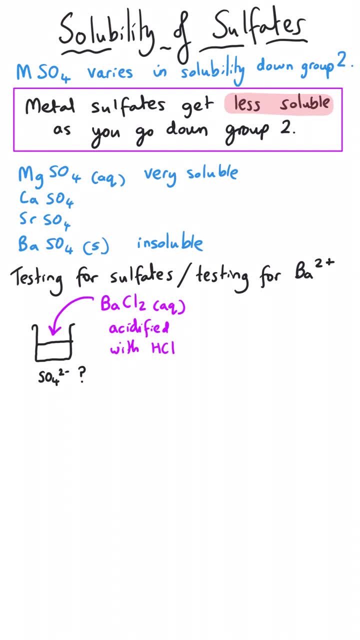 which is usually acidified with dilute hydrochloric acid first, And if we get a white precipitate forming, that is an indication that there were sulphate ions present in the sample that we were testing And the precipitate will be barium sulphate And the ionic equation for the formation. 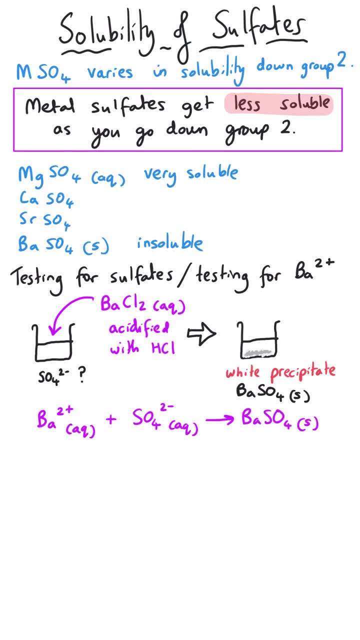 of the barium sulphate. the white precipitate will be barium 2 plus ions, that's from the barium chloride reacts with sulphate ions from the solution that we were testing and turns into barium sulphate solid. So the two reactants were aqueous and the product is a solid, This barium sulphate that we 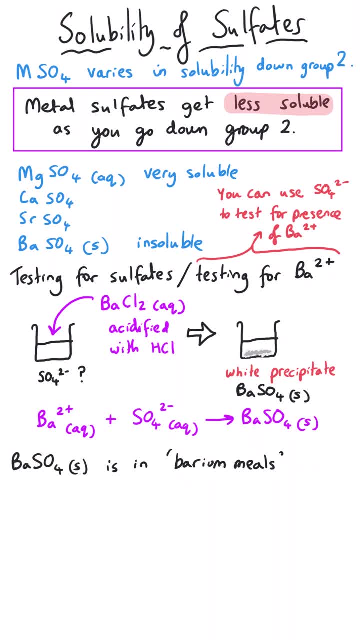 produce is the same chemical that is present in barium meals, And barium sulphate is what's called photo-opaque, And what that means is that when you are in hospital and they're investigating the oesophagus or the stomach or the intestine, what they do is they get you to drink this barium. 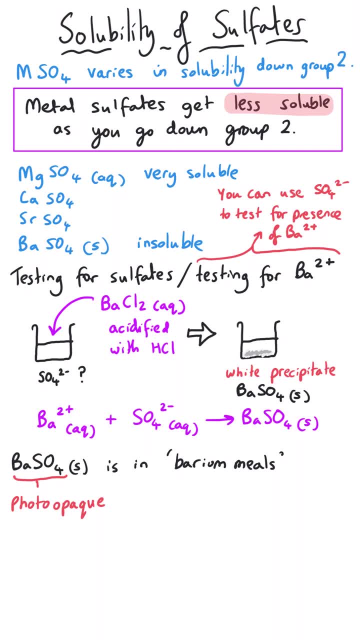 meal which is kind of like thick Gaviscon indigestion remedy in terms of its texture, And what happens is it coats the oesophagus and the intestine, And the x-rays that they fire at you get absorbed by it, And so what you see is: you see the intestine and the digestive tract. 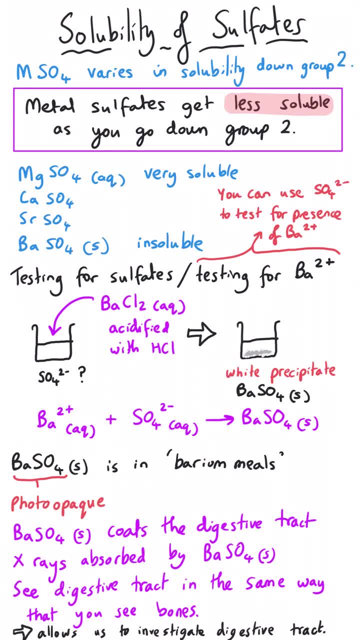 as if it were bone, And that allows the structure of the digestive tract to be investigated in this way. And that wouldn't work if barium sulphate was soluble. The fact is, insoluble allows this formation of a suspension, this barium meal, and therefore allows us to 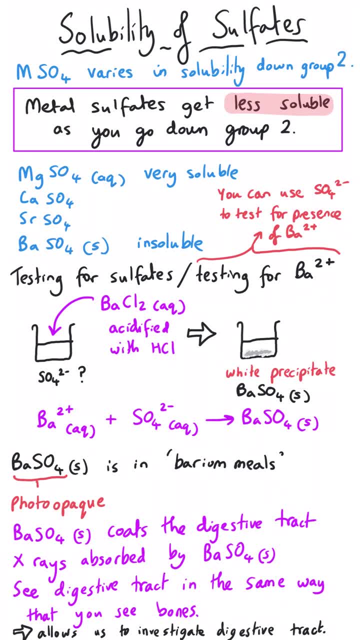 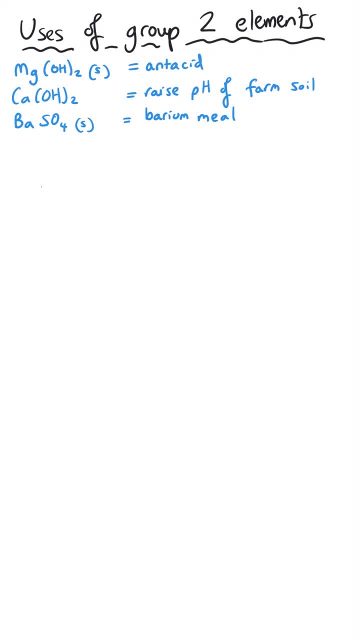 utilise how it interacts with the x-rays. We've seen that group two elements can be used as barium meals during medical procedures, as methods of neutralising stomach acid with magnesium hydroxide and also ways of raising the pH of soil with calcium hydroxide. There are a few other uses. 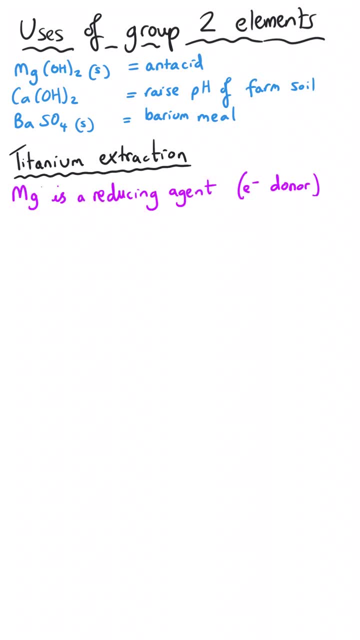 that you need to know. Firstly, you need to know that barium sulphate is a substance that is used as a reducing agent, And that's when the magnesium gets involved. The magnesium acts as a reducing agent by donating electrons to the titanium, And the magnesium ends up producing. 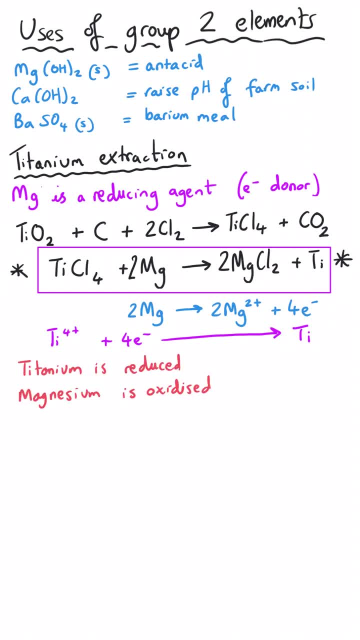 magnesium chloride, which is where the magnesium becomes a two plus ion. This chemical reacts as a reducing agent by donating electrons to the titanium, And that's when the magnesium reacts as a reducing agent, And that's when the magnesium ends up producing magnesium chloride. 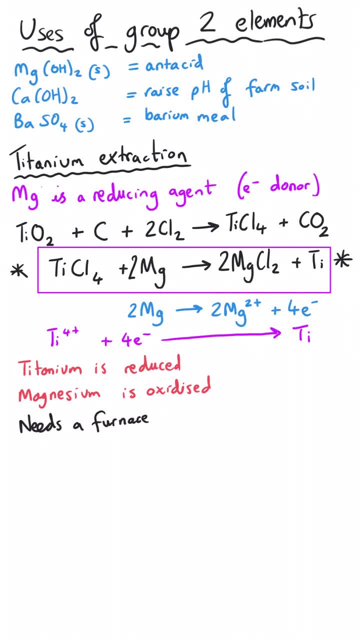 The reaction doesn't happen readily. It takes place in a furnace at almost a thousand degrees C, so it has a high energy demand to carry it out. The final use I want to talk about is the removal of sulphur dioxide in flue gas from things such as power stations. You will know that sulphur 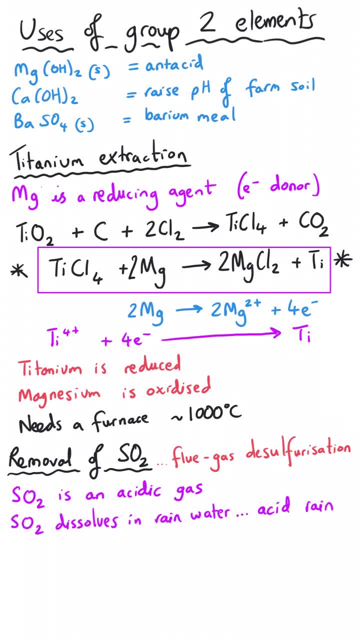 dioxide is an acidic gas which, when dissolved in moisture in the air, can contribute to acid rain, And so it's very important that we try to limit the release of sulphur dioxide into the atmosphere. To do this, we use group two elements: calcium, specifically in the form of calcium oxide, or 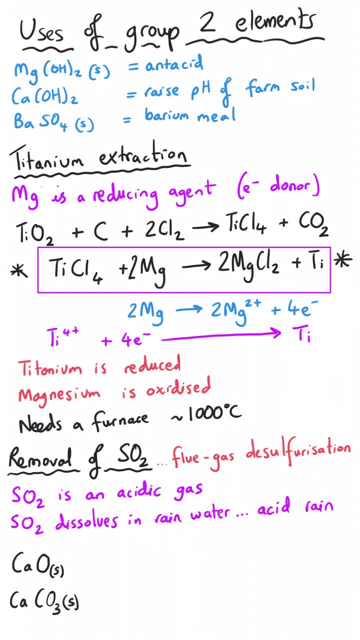 calcium carbonate, usually from the same source- limestone. So calcium carbonate is the chemical name for limestone, and calcium oxide can be derived from limestone in a thermal decomposition reaction, And so the sulphur dioxide can either react with calcium oxide and water to produce calcium sulphite, which is C-A-S-O-R-B-I-C-O-R-B-I-C-O-R-B-I-C-O-R-B-I-C-O-R-B-I-C-O-R-B-I-C-O-R-B. 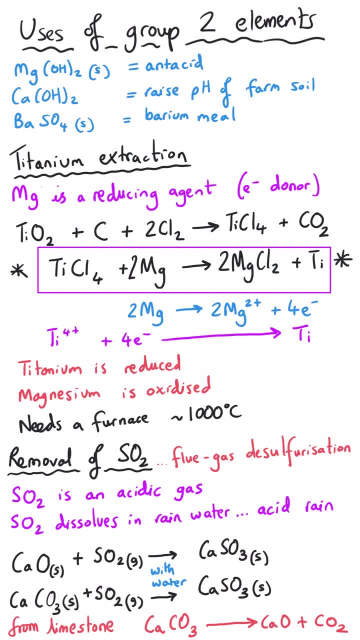 Or it could react with again water and the calcium carbonate, again producing the calcium sulphite and also water and carbon dioxide. Clearly, both of these processes are beneficial because we don't contribute to acid rain, but both of them have some problems. 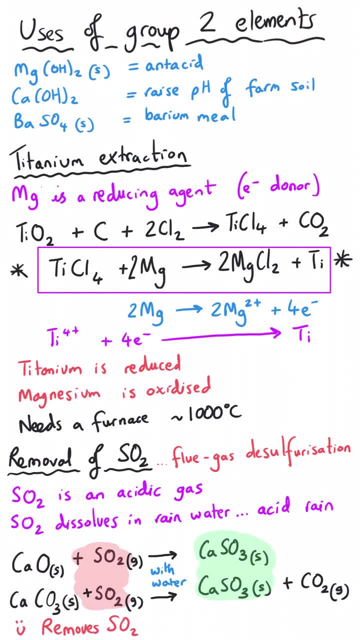 For instance, both of them produce calcium sulphite. So where do we put this solid waste product that has been produced? Do we put it into a landfill, Because that will obviously contribute to a negative impact on the environment. We don't have limitless space to do this. 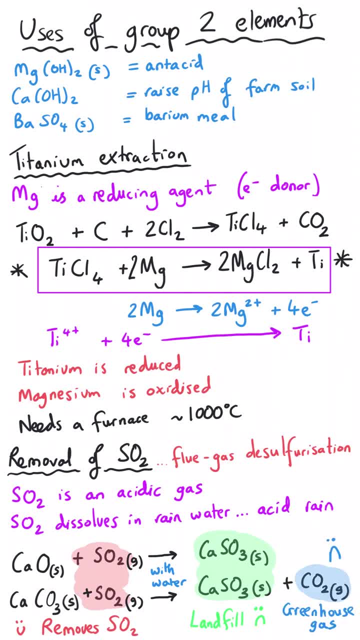 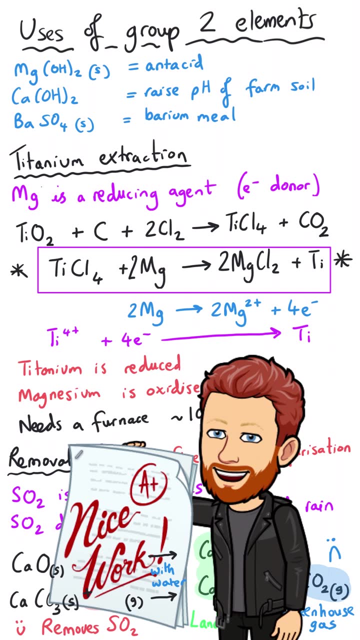 The second method is even worse, because not only do we have that issue, we also produce carbon dioxide, which, as we know, can contribute to the greenhouse effect because it is a greenhouse gas. Okay, that's the end of this video about group 2 metals. I hope it was useful.